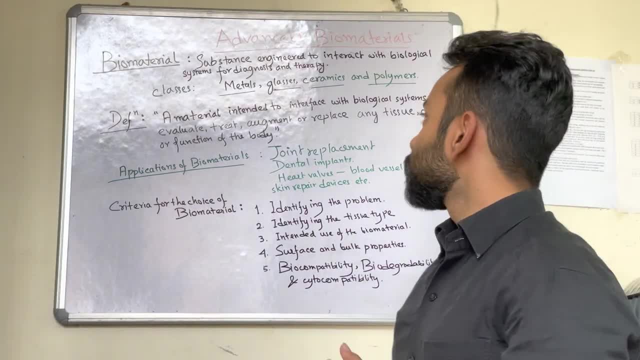 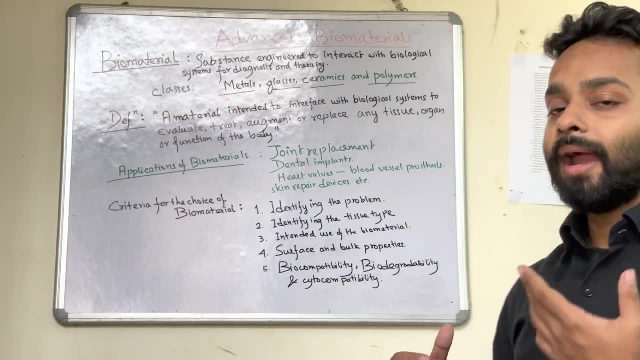 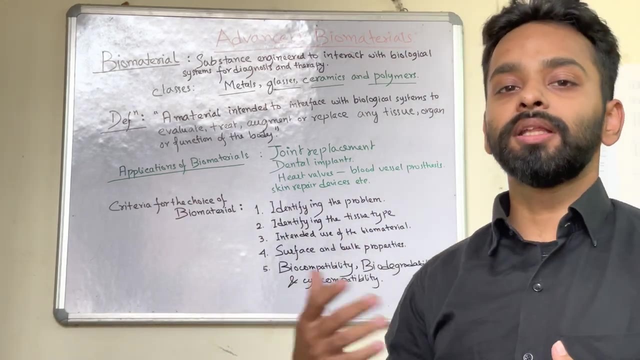 So biomaterial is any substance which is engineered to interact with a biological system for diagnosis and for therapy. Now, these biomaterials can be used either individually or individually. These biomaterials are usually used with a few different purposes or in combination with other such materials or systems. so there basically. 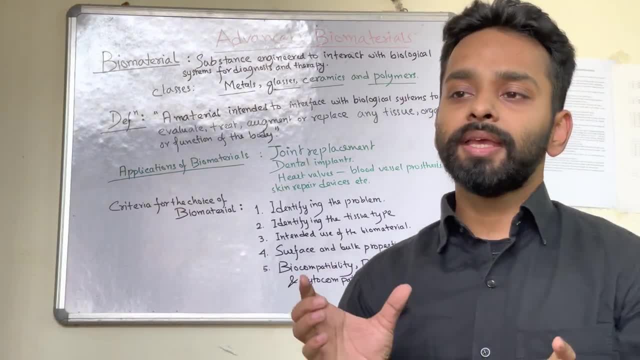 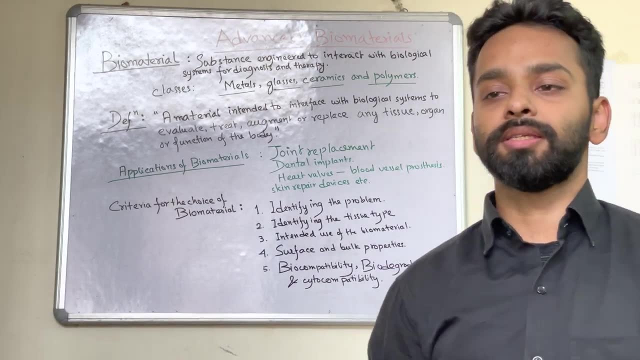 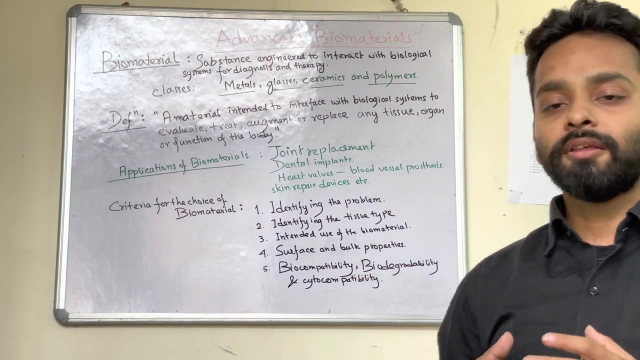 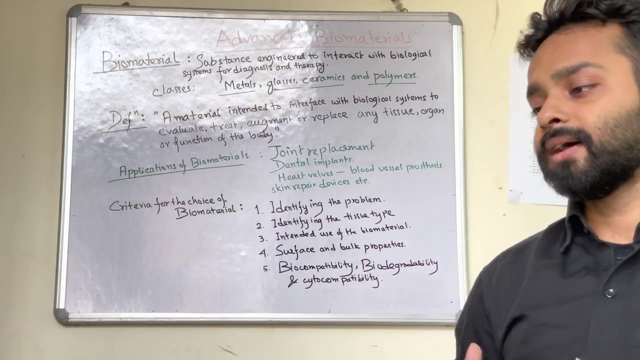 if we want to summarize just a, biomaterial is any material which is intended for uses in direct combination with biological systems. so such biomaterials can be divided into four main classes. the first class is metals. now, the metals are the sum of. are the examples which are one of the most 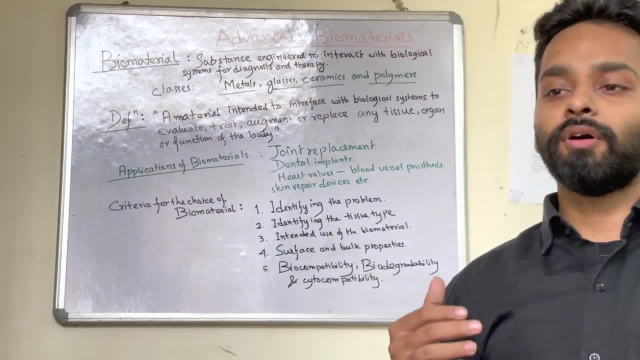 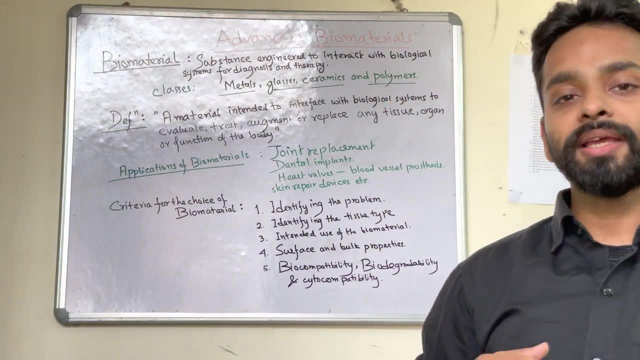 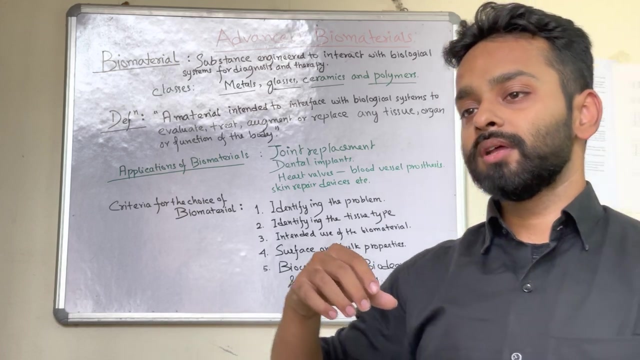 primitively used material for direct in use with a human body, for example, the most prime example is the dental implants. so now, initially, when people used to lose their teeth, they used to resubstitute it with black, gold or silver implants. so that was the first class, and the second class are the metals. 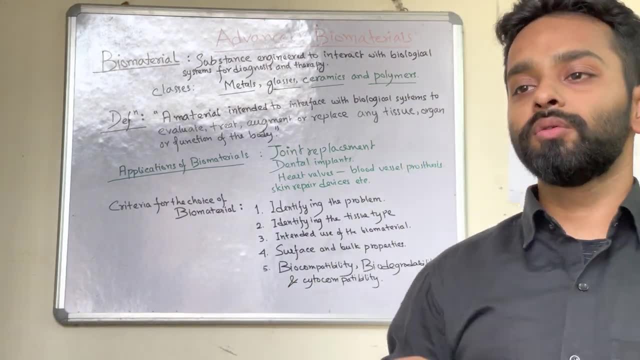 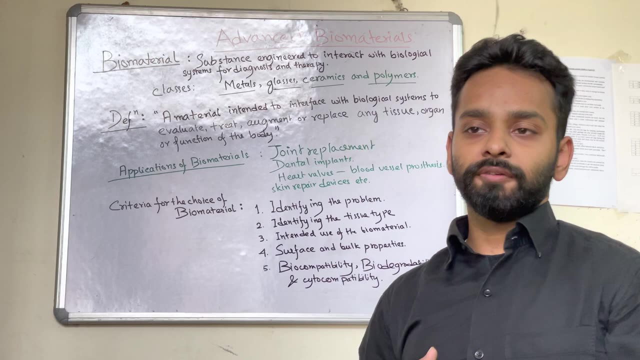 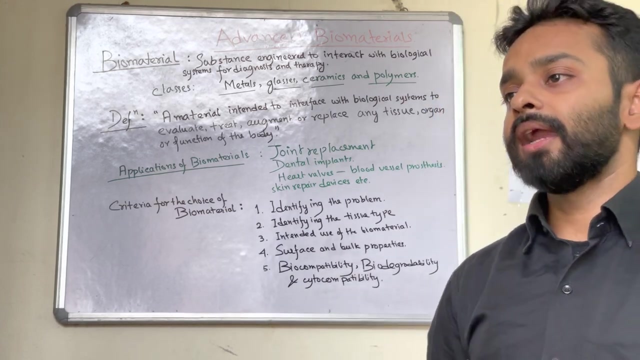 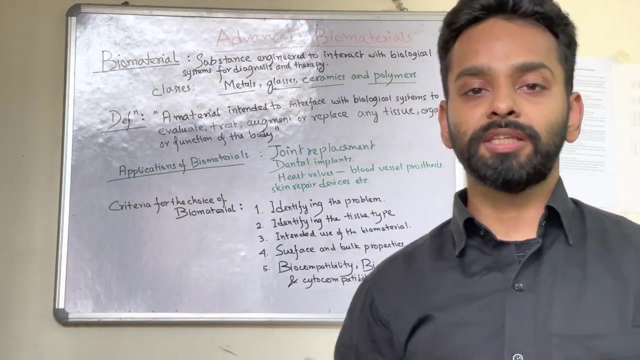 the first time when metals were used in a human body to serve a particular function or give an aesthetic value. but now, with the development of science, these metals find their applications in different fields of biomaterial, biomedical engineering and tissue engineering as well. so now when hip arthroplasty or shoulder arthroplasty, or in placement, 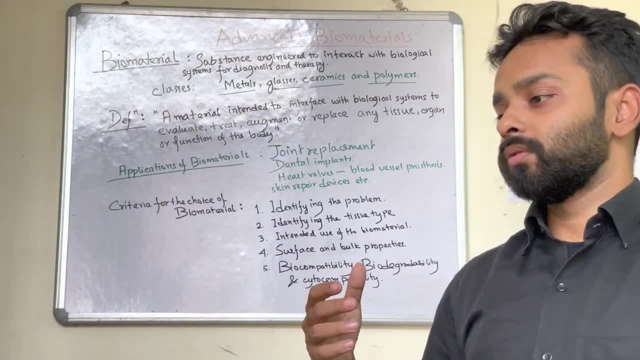 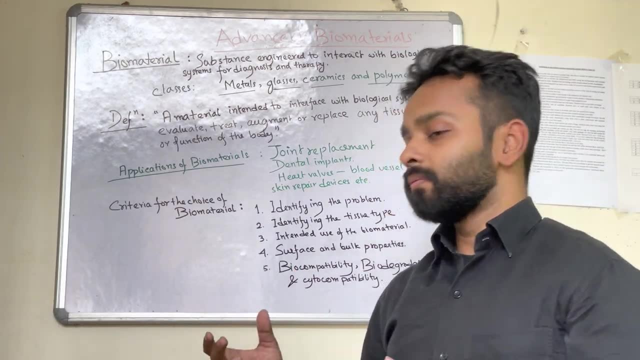 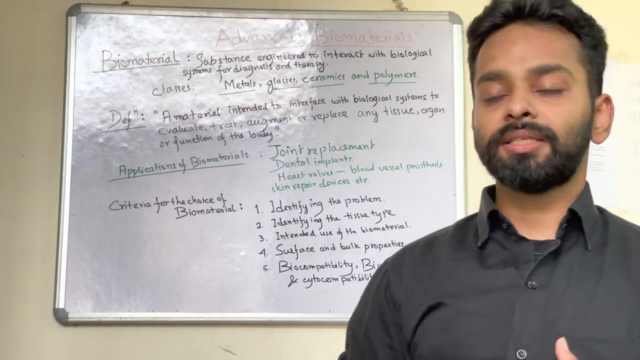 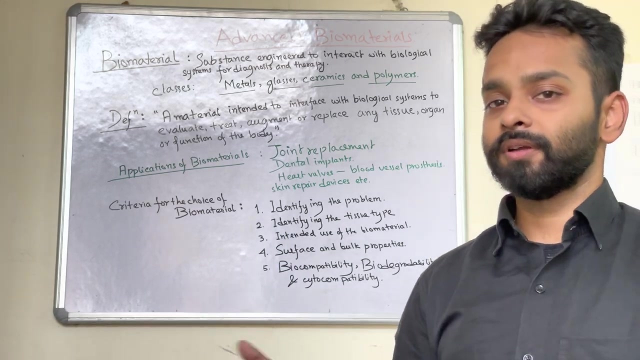 surgeries are done with both tissues. so metals are mainly used, used as plates, as you know, as stents. so metals find their application in different fields in biomedical engineering because of their inert nature and also their malleability, ductility, and you know, their fabrication into different shapes as well, so for different joint replacement. 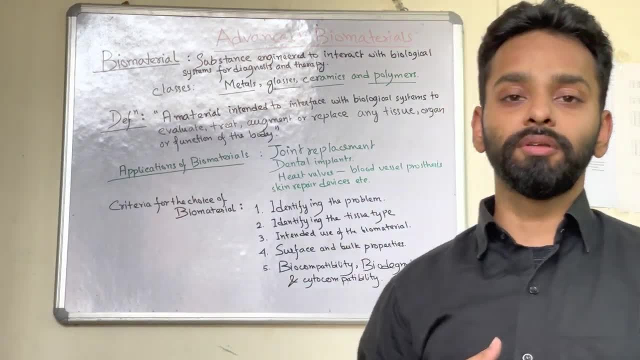 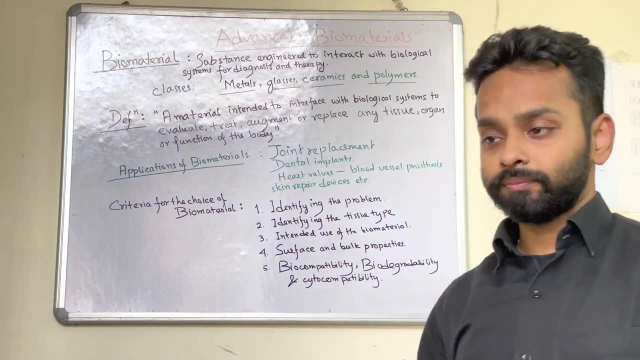 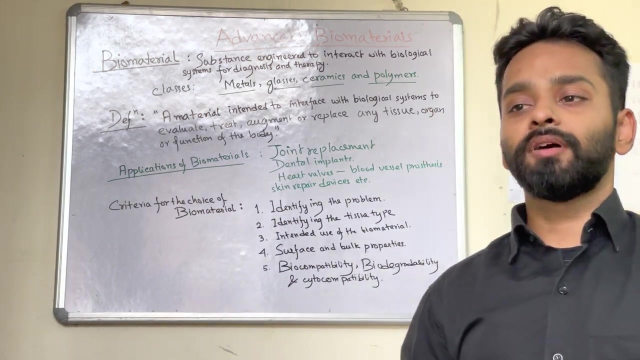 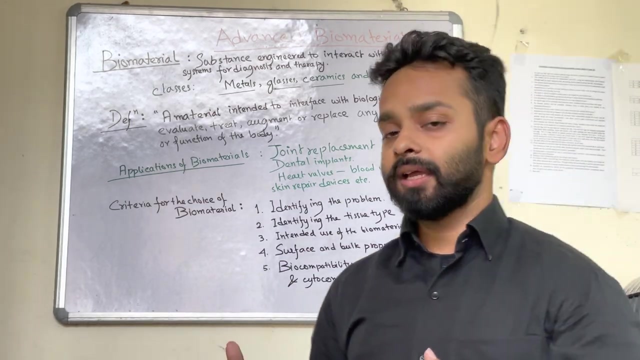 surgeries. initially, metals was the most important choice for any scientist. so metals can either be used individually or in order to improve their properties. they can be used as alloys. so alloying is amalgamation of more, one or more than one metals to improve their physical properties. so there are specific alloys. 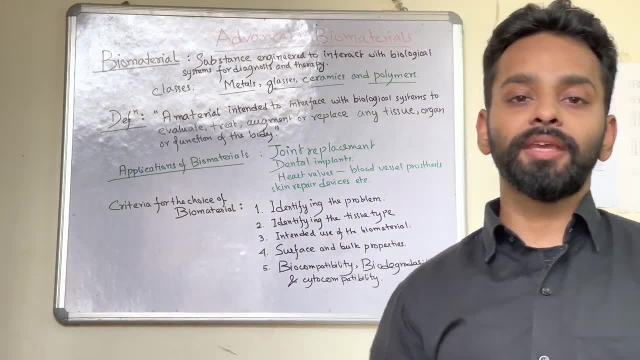 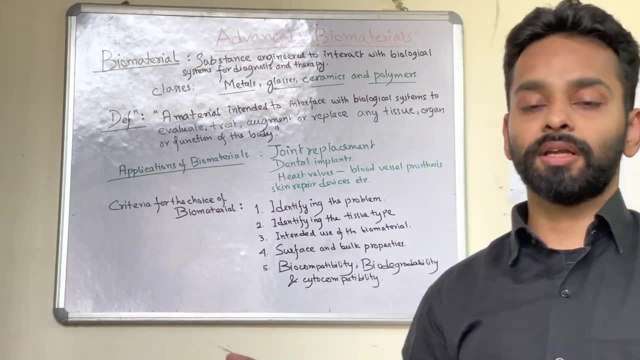 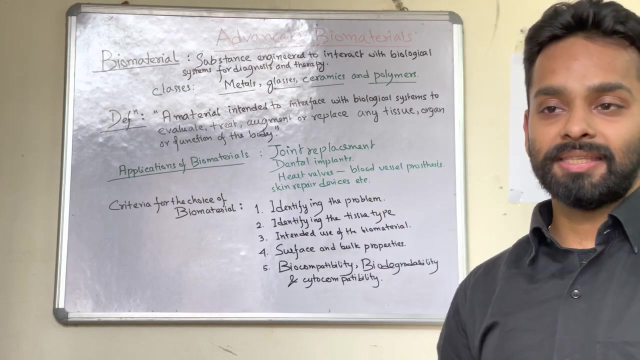 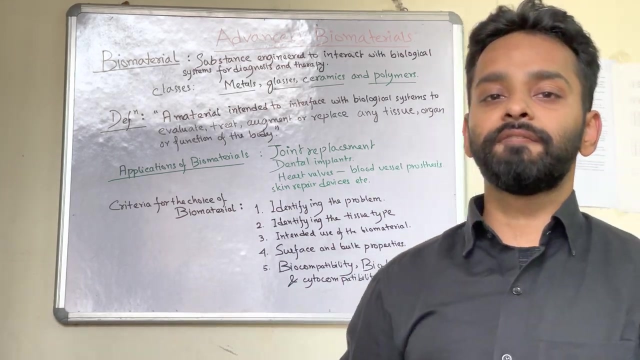 such as nitinol, which is mainly used in manufacturing stents or valve prosthesis and also for making stents for correcting atherosclerotic artery diseases. also, there are titanium, aluminium, vanadium, alloy, stainless steel, you know, and many of such examples are there, which find their applications in different fields of tissue engineering and 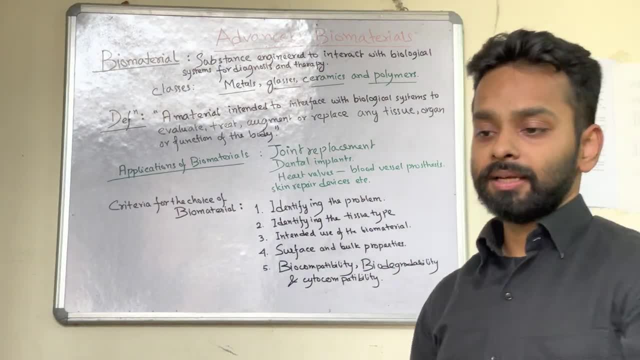 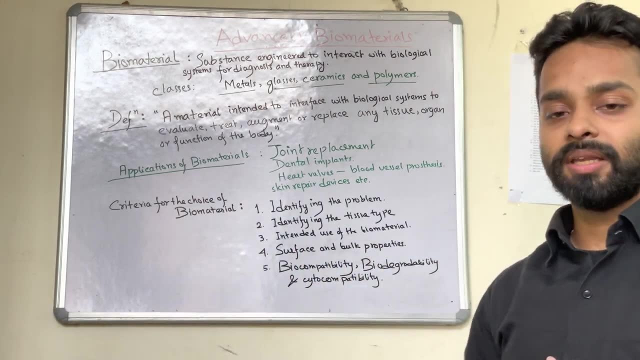 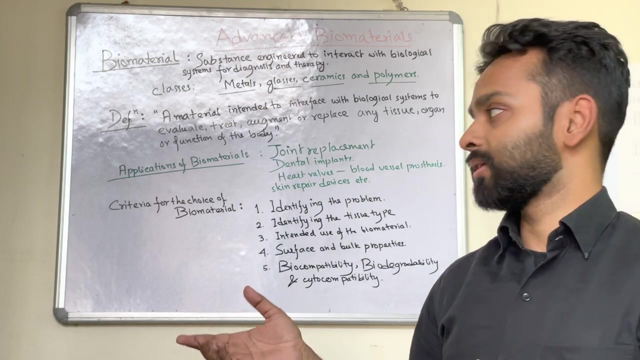 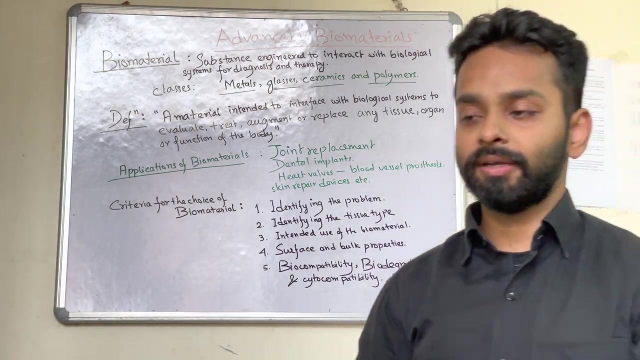 biomedical. the second class is the glasses. the glasses are the silica based compounds, so their main role is in the ocular replacements or in the correcting of different ocular diseases, so making lenses implanting. so these were usually done with glasses. the third category is an important criteria of biomedical biomaterial, which are ceramics. now these ceramics have 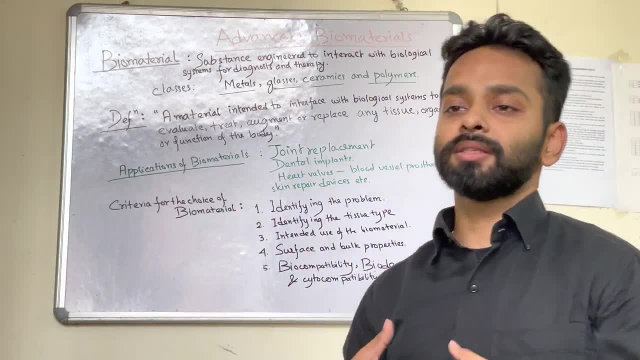 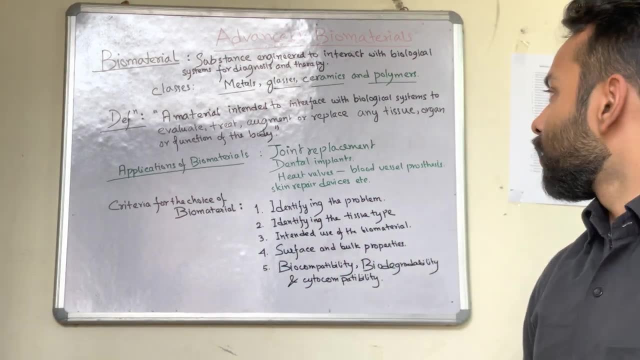 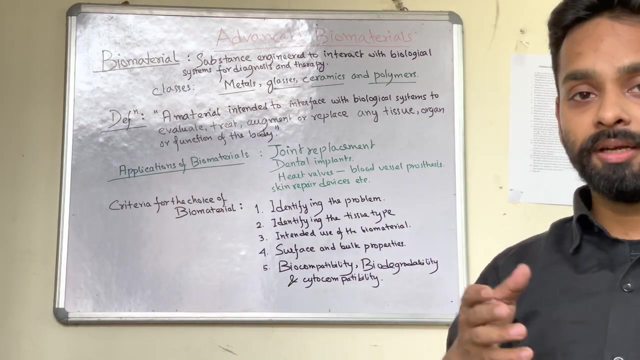 properties which are different from that of metals, so ceramics. examples include hydroxyapatite, which is a calcium based ceramics. alumina, aluminium oxide does our alumina. all these are ceramics. now their ceramics are also finding the roles in different arthroplasties and in different bone, in tissue engineering approaches and joint replacements. 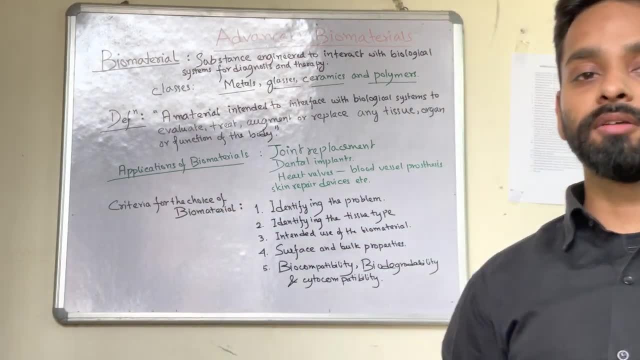 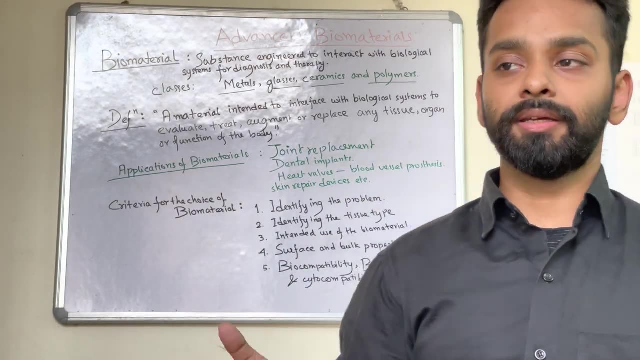 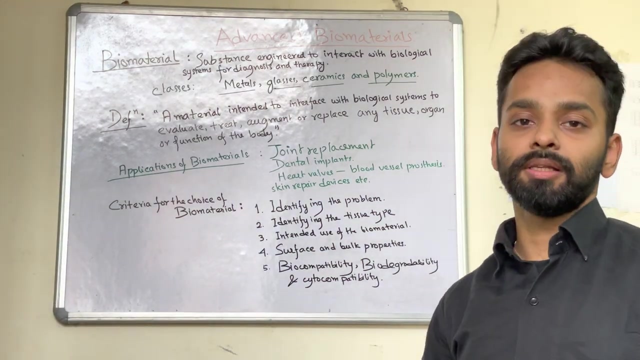 because ceramics show an individual unique property of much greater, better hardness, surface properties and also much lesser wear and tear when used in multiple cycles. so ceramics are also finding applications in different fields of tissue engineering and biomedical engineering as well. and finally, one of the most important classes of biomaterials. 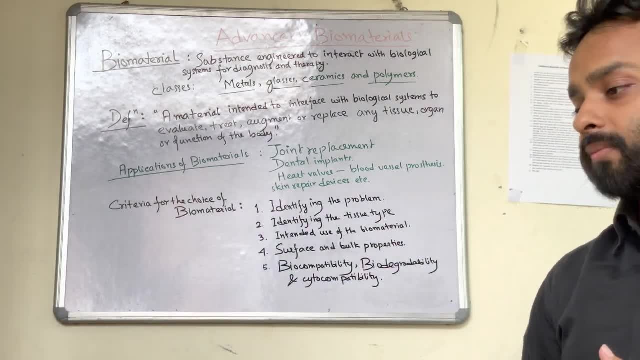 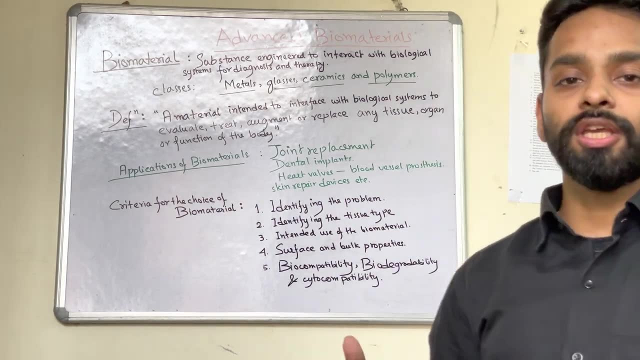 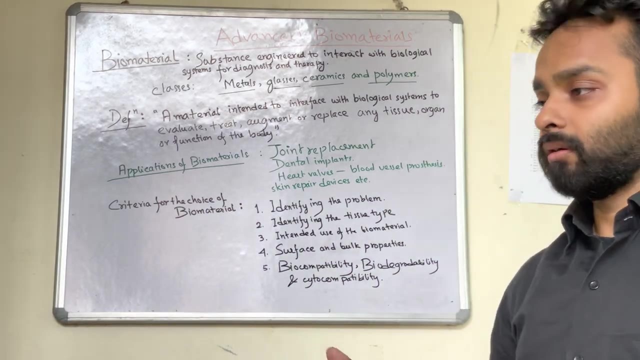 which are coming into light are or have been used for quite some time now. since are the polymers. now, these polymers are a class of materials which have very unique properties. so polymers are basically repeating units of a particular material or an analyte of a material which can be natural or 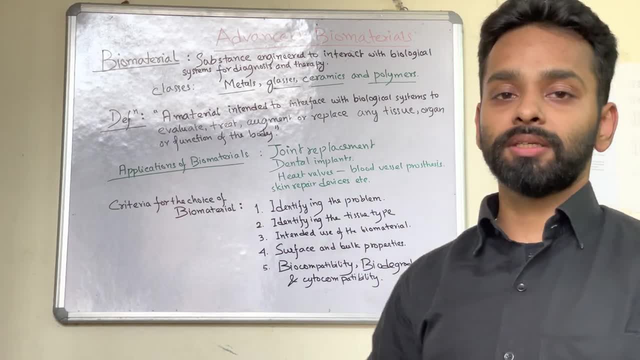 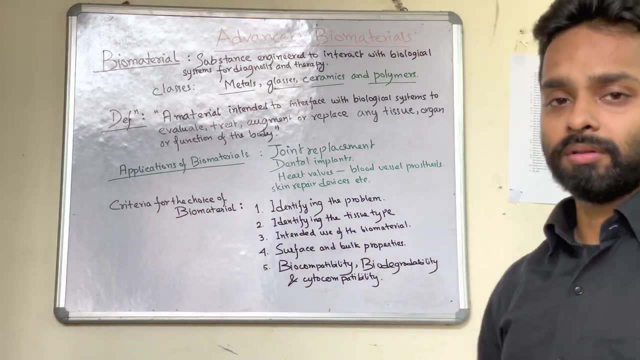 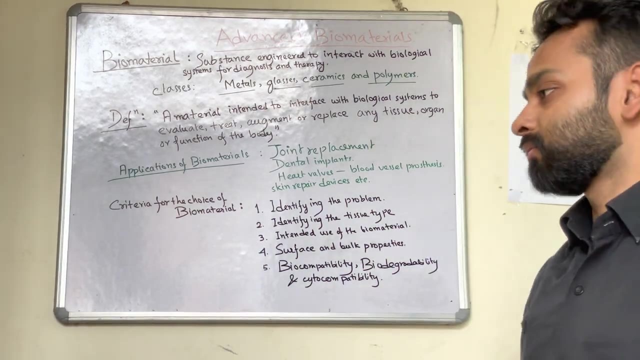 synthetic natural polymers. examples include the polymers of the material, called polymers of the soil up. so Polymer examples include collagen, starch, celulose, chitosan and many others. all the protein based on polymers are the natural types of polymers, such as silk, fibroin. all these polymers are natural and the various types of synthetic polymers include the polyhenyl alcohols, the poly-anisocorpyle acrylic inite and the acrylic acid based polymers and many other types of phases like merende. such polymers exist Now. with using polymers in combination with each other, it is possible. 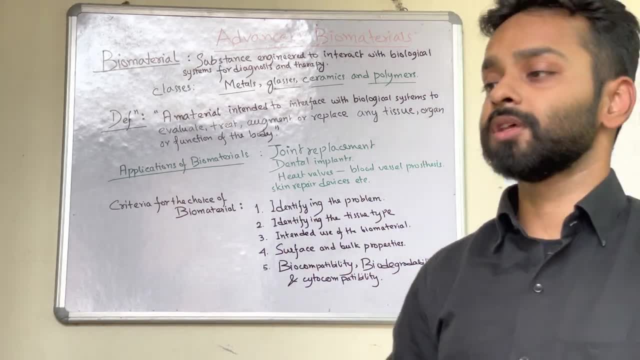 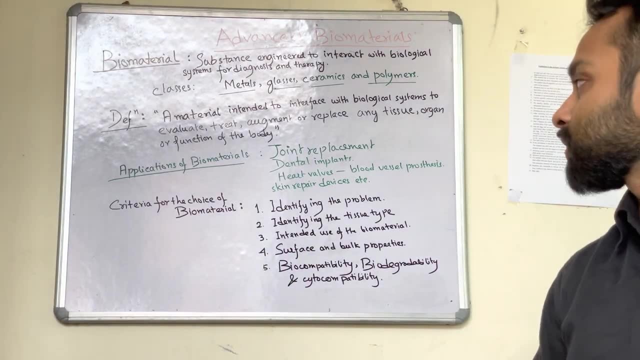 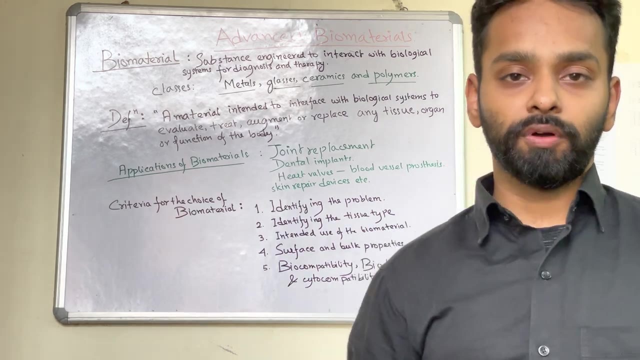 to fabricate different types of composite polymeric systems with different properties which can be tailored to suit a particular requirement in tissue engineering approaches. So, after looking at these examples, so now if we try to make a working definition of what a biomaterial is, so it would summarize as a material which is intended to interface. 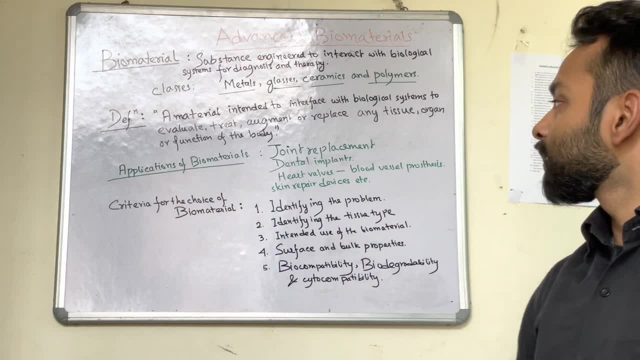 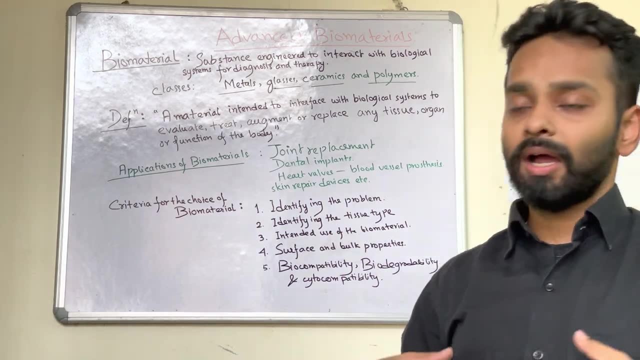 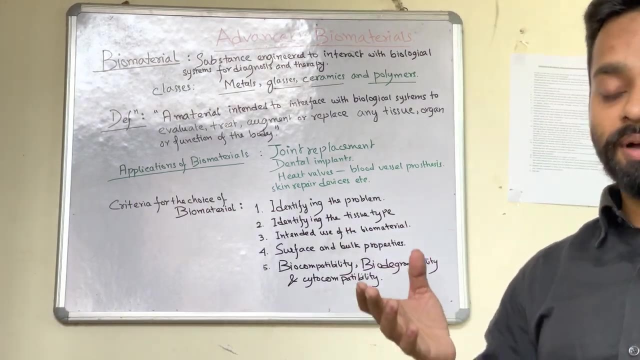 with biological systems to evaluate, treat, augment or replace any tissue, organ or function of the body. So after this, what are the different fields in which these biomedicals can find their applications? So these biomedical biomaterials can be used for fabricating different 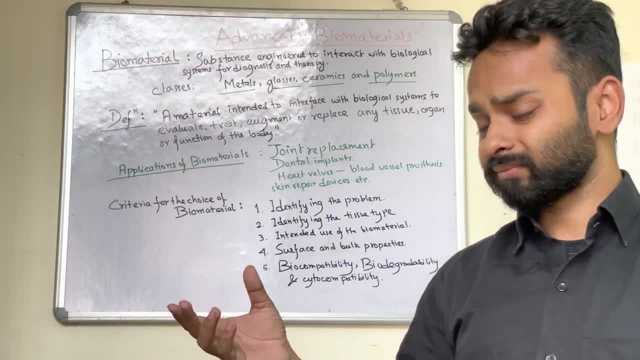 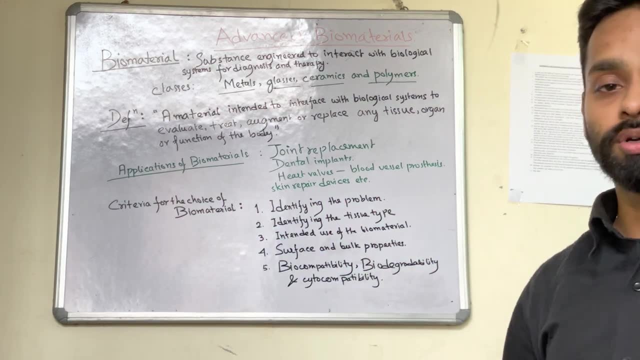 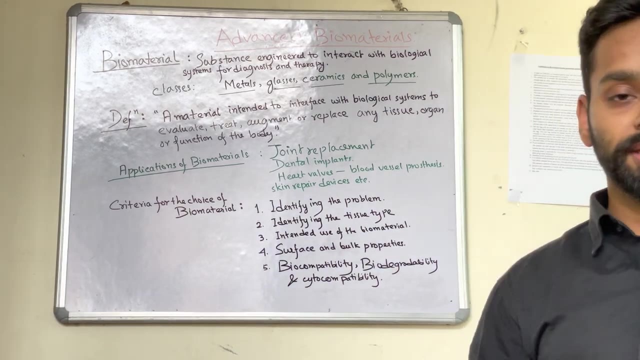 devices or different materials, For example the composite materials for their roles in hip joint replacements, such as the shoulder joint, the hip joint replacement surgeries, the arthroplasties, tendon and ligament repairs, dental implants and dental fixatures, then the heart valve prosthesis. 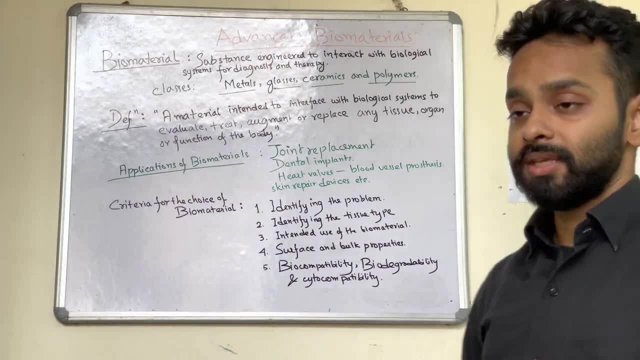 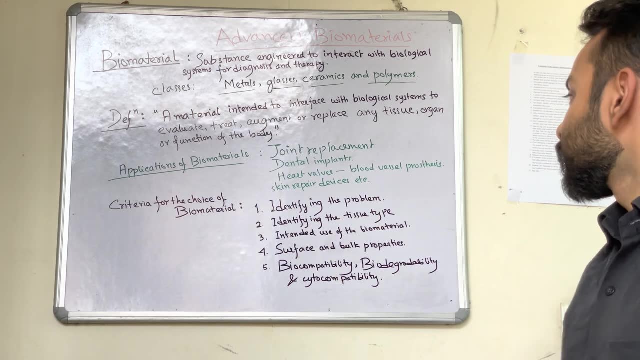 the vessel prosthesis as well. So different skin repair templates which we will be looking at in great detail in the upcoming lectures. So there are many different types of biomaterials. There are many such examples where these biomedical biomaterials can be used to fabricate. 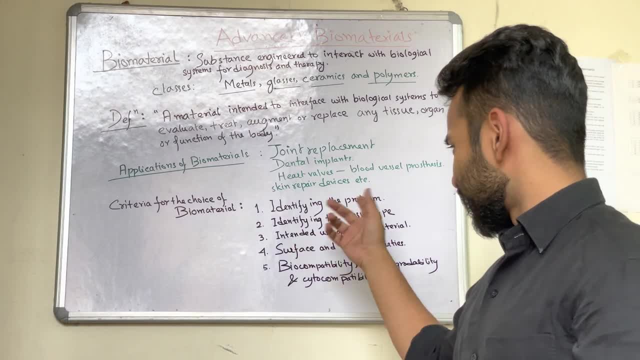 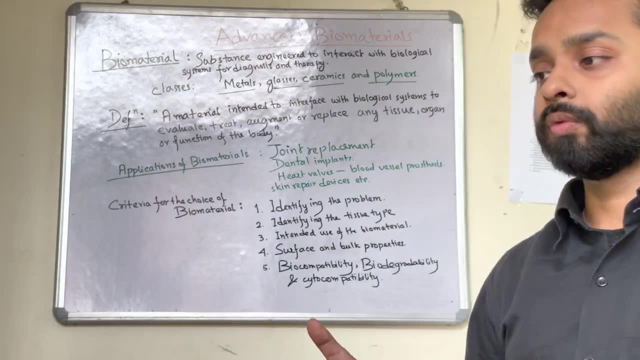 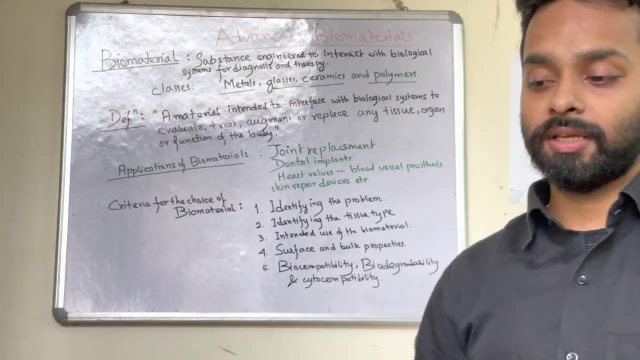 So if we discuss one particular example, such as a skin repair device, so this would essentially imply a system which can actually consist of two composite polymers- Now they can be natural, such as type 1 collagen and chondroitin 6-sulfate- to provide the two. 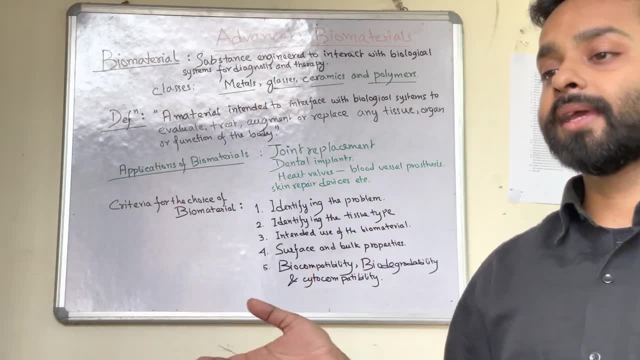 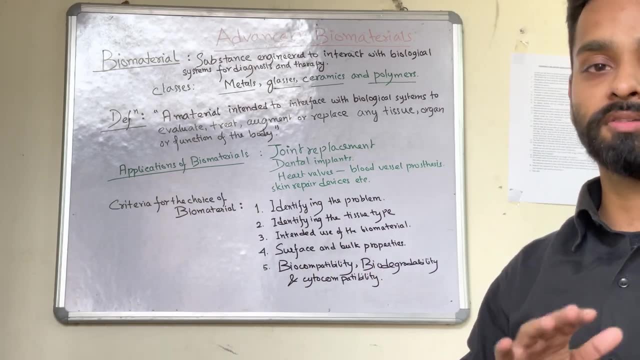 layers for the dermis and epidermis, Dermis and epidermis repair, And they can also be fabricated in form of a scaffold, which is a three-dimensional mesh-like network structure, a crosslink structure which has pores for migrating, migration of different. 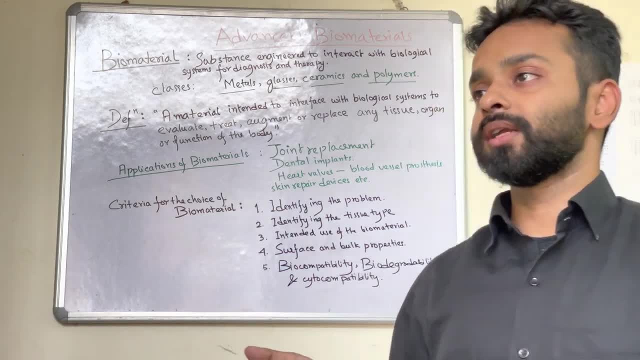 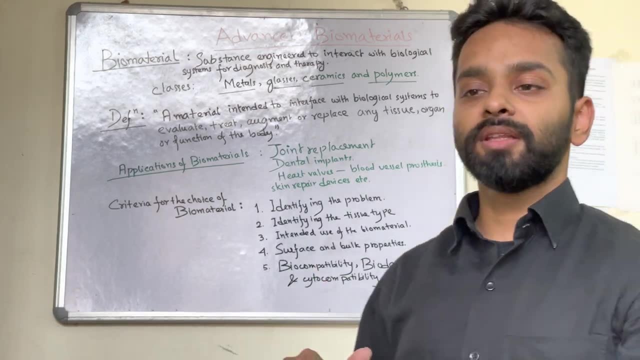 cells when they can be seeded with it. So basically, what it is done is, after fabricating that scaffold, they are seeded with cells. These cells are mainly the fibroblasts. So after seeding with the cells, they are taken and implanted into an area with a large.